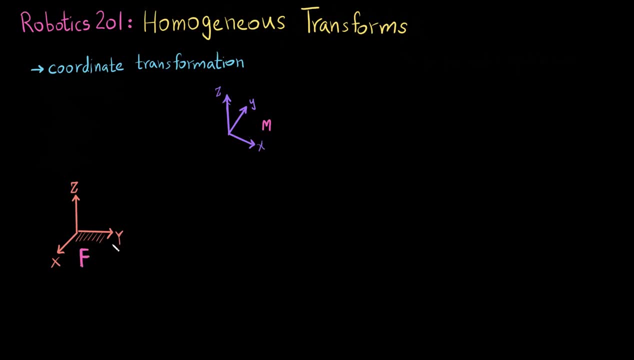 is the fixed reference frame. so the question is: how do I express the moving reference frame with respect to the fixed reference frame? that is, what coordinate transformations is. you express one coordinate system with respect to another coordinate system. but before we get into how we do that, we 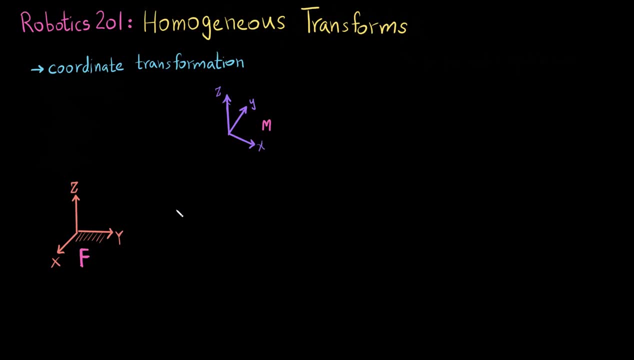 need to understand why do we need to do all the Hesse and do coordinate transformations in the first place, right? so in order to understand that, let's see, I have a robot which let me draw something out. my my drawing isn't that good, but let me try my best. so I have a. 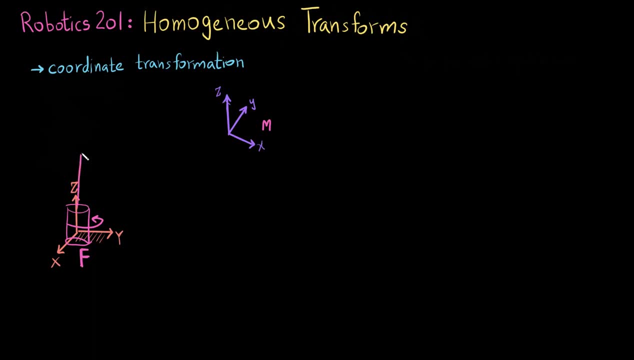 robot which has a base which can rotate about this and then do is another joint here which can rotate about this and it is connected to another join which is that's a prismatic joint and which is connected to the gripper or the end effector. so what I've 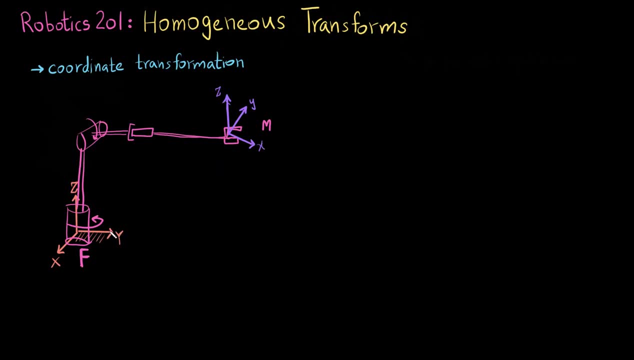 done is I have. so what I've done is I have fixed the fixed reference frame at the base of the robot and the moving reference frame at the end effector of the robot. so that is why I need to coordinate transformations, to be able to identify where my end effector is at any given time. 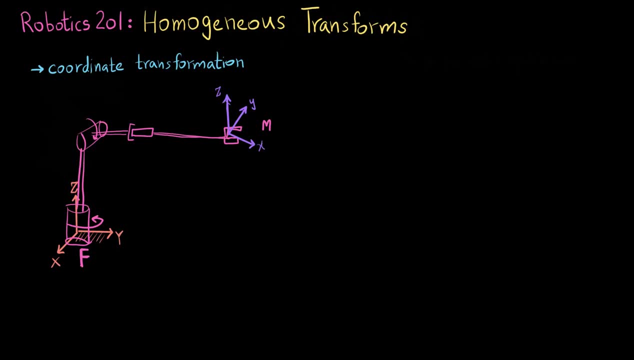 hope that makes sense. so how do I do it? so, first and foremost, you can see that in order to go from the fixed reference frame to the moving reference frame, you need to do some translation right, and for this case, you need to translate first about X by a. 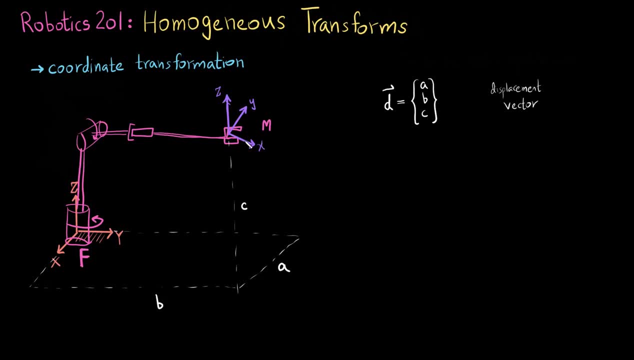 unit, then by B units in y and by C units in Z, as represented by this displacement vector. so you first displace the fixed frame by this displacement vector to get to this point. however, notice that even once you reach this point, your orientation is not aligned with the moving frame. right. 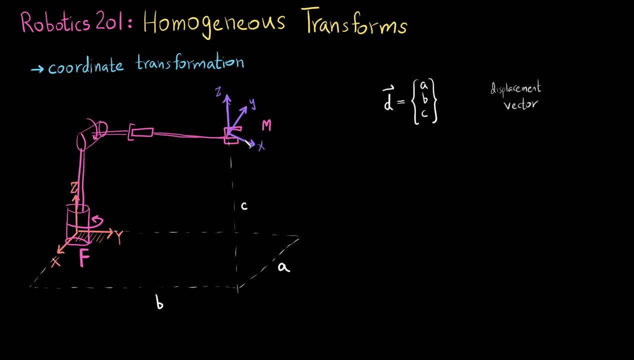 so you need to do a rotation in order to get your orientation aligned with the moving frame. for this case, if I can just quickly see that, what would happen is, once I do that, the displacement what I would get is I would probably get: my Z axis would be aligned with the z-axis, my x-axis would be here, right. so what? I? 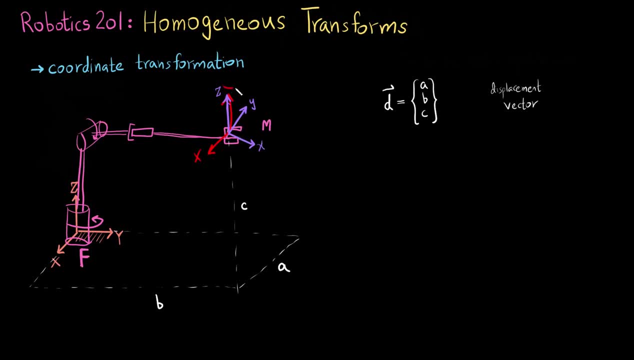 would do is I would then need to do a positive rotation about the z-axis by whatever this angle is, so theta, in order to get this aligned, and what that would mean is that would ensure that my moving frame is now expressed with respect to the fixed frame. so you see that there are two things that I need. one is a. 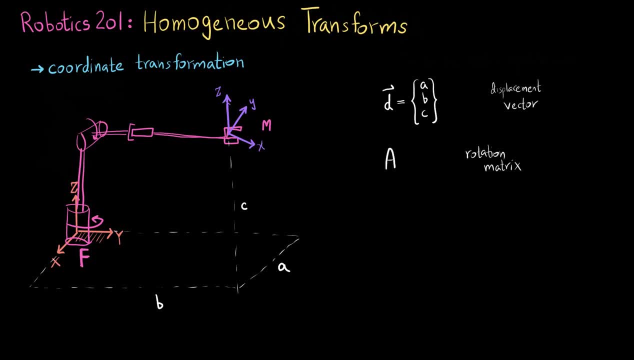 displacement vector and the other is a displacement vector and the other is a rotation which we normally represent by the letter A, which is called a rotation matrix. so there is a rotation matrix and there is a displacement vector. now let's say I have a point X which is expressed in the moving frame. so let's say there is 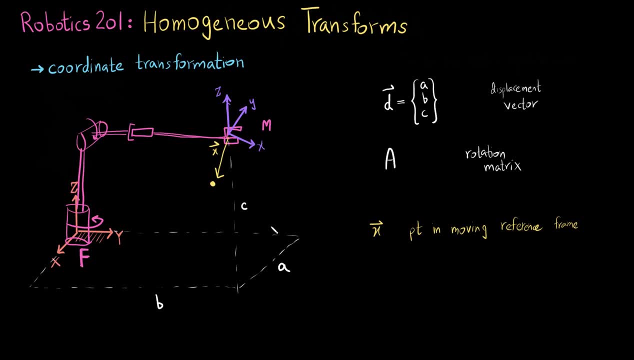 an object that the robot needs to grab, and we know the position of the object with respect to the end effector. so which is a small x? now we need to figure out the position of that same object with respect to the base of the robot, with respect to the fifth frame. so I have 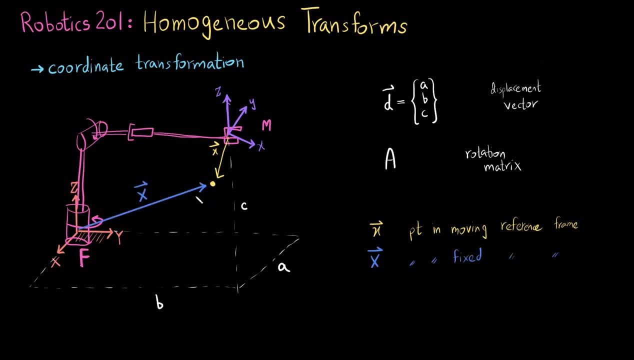 marked this with capital X, and that is often the case that we need to do. we need to find the position of one object with respect to two different frames: respect to the base of the robot, with respect to the end effector of the robot, and sometimes even respect to the end of the room or something. so, when talking, about a point with by a constant space vector andupun duplicate vector with respect to a part next to the mezieth frame, and we will learn a lot about an object shape and will learn equations as to how different ones can be formed in a general center positive set. 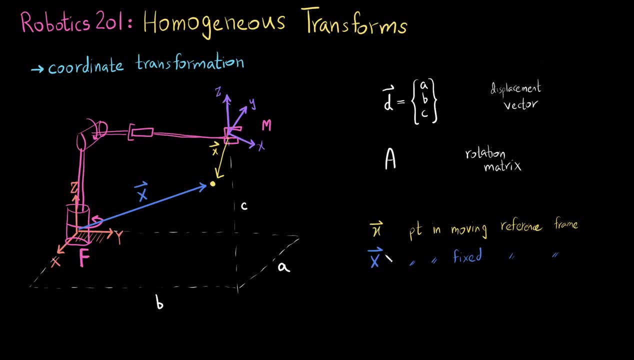 with respect to the moving frame, we use small editors. when talking about the point with respect to the fixed frame, we use capital letters. that is just a convention. so how do we express the same point, expressing the moving frame to the fixed frame? so the way is very, very simple. this is: 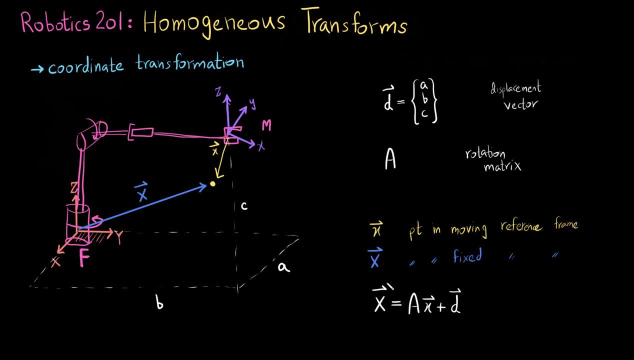 what coordinate transformations is. so what you do is you use this equation right here, which is: big x equals to the rotation matrix times the small x plus d. so this is the equation that we use. but what does this equation mean? let us try and dissect this equation a bit. so, first and foremost, you can see, if you look at the second term here, you can see: 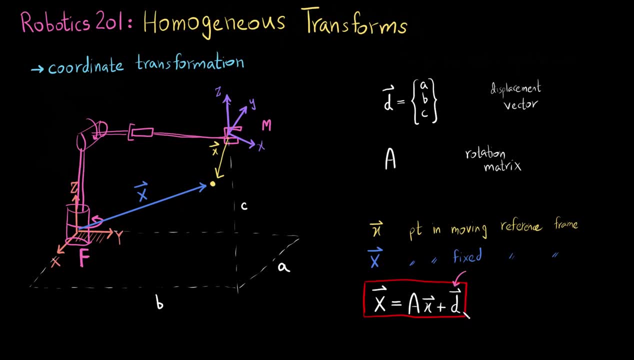 that what you are doing is you are first displacing it by the displacement vector, which makes sense, which is what we did initially. we displaced the fixed frame by the displacement vector and then you are multiplying the rotation matrix with the point. so you multiply the rotation matrix with. 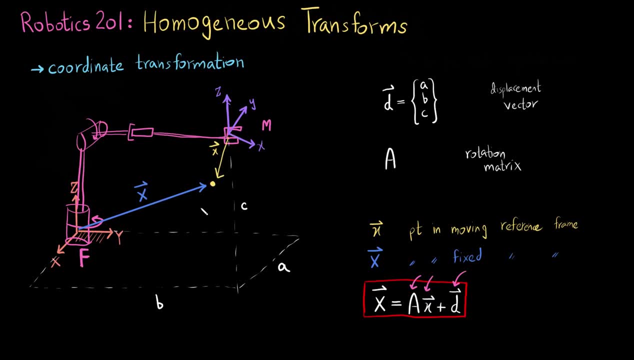 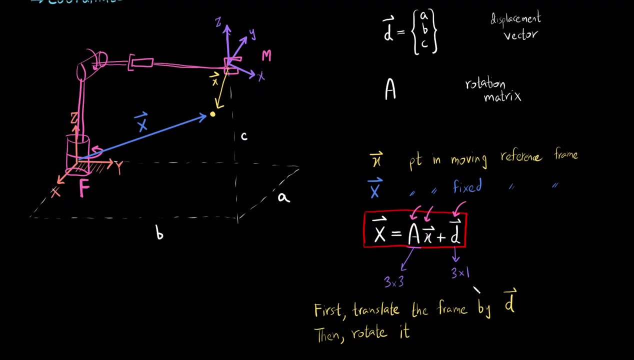 the point okay, which gives you the same point expressed in the fixed frame hope. that makes intuitive sense and it the way that you read this is. you first translate the frame by the displacement vector and then you rotate it, so it's reading from right to left and the displacement vector is just a. 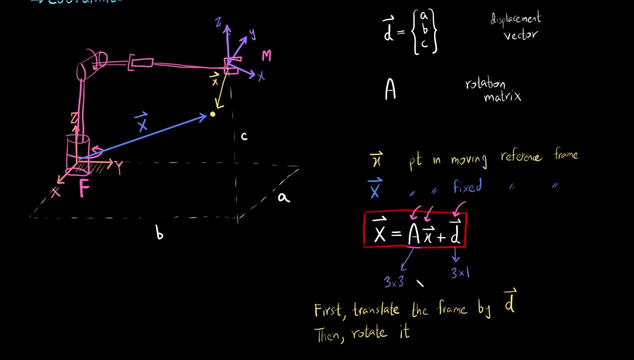 vector, which is 3 cross 1, and the rotation matrix is a 3 cross 3 vector, and we have talked a great amount about the rotation matrix in our previous video. so the rotation matrix is a 3 cross 3 vector. the displacement vector is a 3 cross 1 vector and this is what coordinate transformation is. 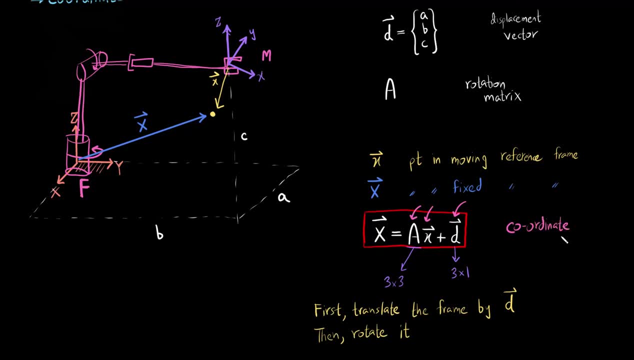 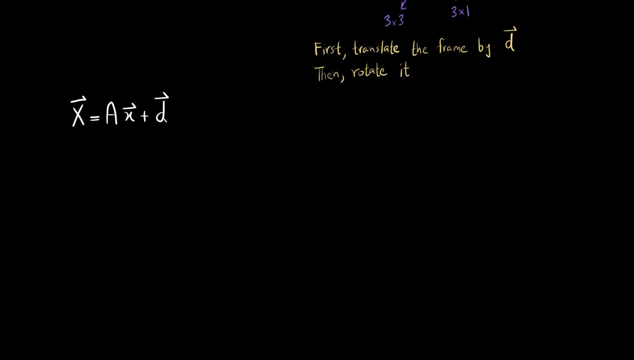 so you are expressing a point and with respect to one coordinate system, and like a point defined with respect to one coordinate system, and you are expressing it with respect to another coordinate system. so, coordinate transformations now. now i've read it in this equation and what what we do often is we do not want to have two separate. 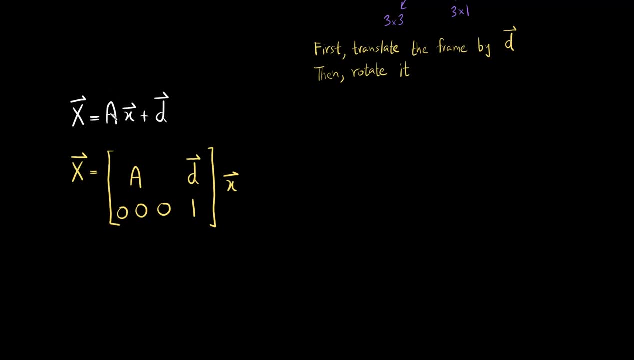 entities, that we have to multiply, that we have to add and get the point. what we do is we combine all of this into one matrix. so the way we do it is, we make this matrix, which is a 4 cross, 4 matrix, and on the top left side we 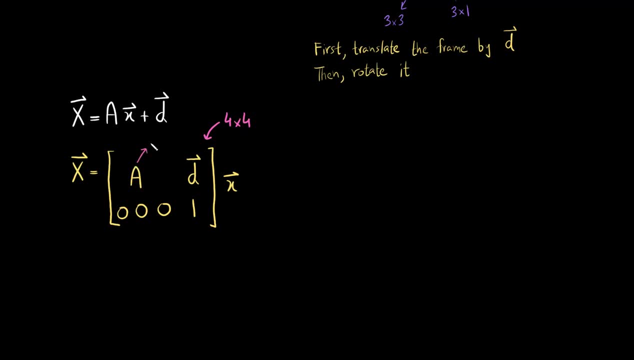 keep the rotation matrix, so it is a 3 cross 3 matrix. and at the bottom of this matrix we have three. we keep three zeros. that is always the case. and on the right side we keep the displacement vector, which is a 3 cross 1 vector. 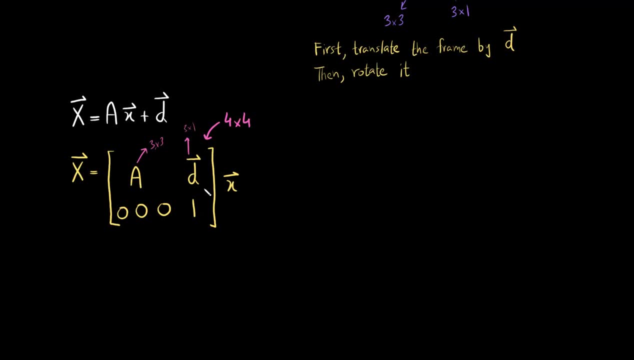 and at the bottom we keep a 1. so it's just combining the rotation matrix and the displacement vector together, and for the bottom row we just use three zeros and a one. so now we have a 4 cross 1 and we multiply it by small x and we get the capital x. but wait, if this is a 4 cross 1. 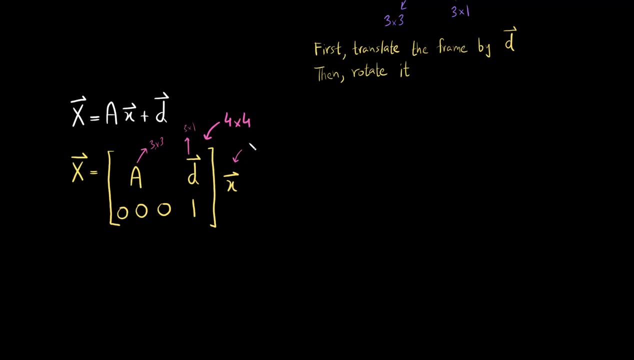 matrix, then this cannot be a 3 cross, 1 vector, right, because it cannot be multiplied. and, yes, that is exactly the case. so when we are using this specific form, which is when we have combined the rotation matrix and the displacement vector into one single matrix, so when we are using the same equation, what we do is: 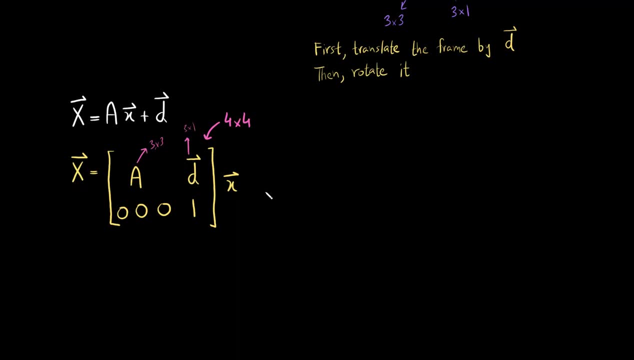 instead of just using the small x and the big x, which is a 3 cross 1 vector, we keep a 1 at the end of both of these, so the small x would be just x, y, z coordinates, followed by a 1 and the big x. 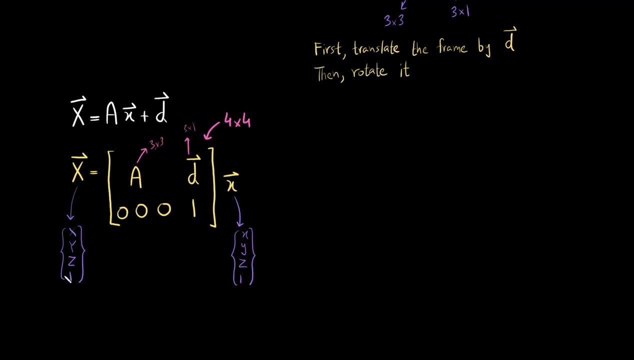 would be x, y, z coordinates followed by a 1. so the 1 is always going to be there, and when we do this, we call this to be the homogeneous point, like the point expressed in the homogeneous form. so this small x is going to be the point expressed in the homogeneous form with respect to the. 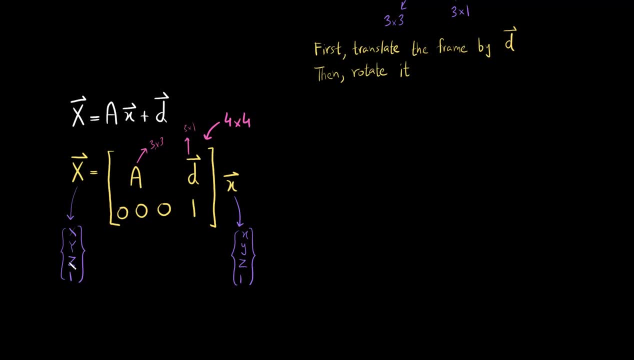 moving frame and the big x is going to be a point expressed in the fixed frame which is in the homogeneous form and this big matrix that we have just made, the 4 cross 4 matrix. this is what we call a homogeneous transformation or a homogeneous matrix, homogeneous. 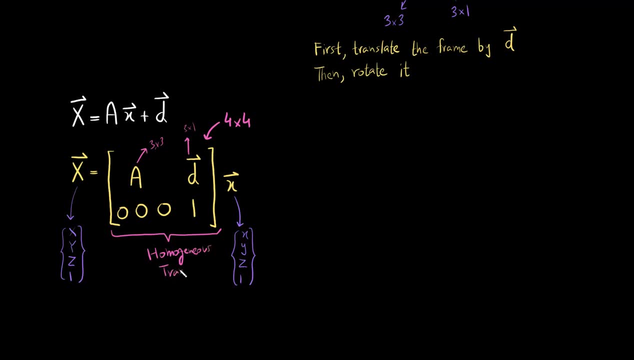 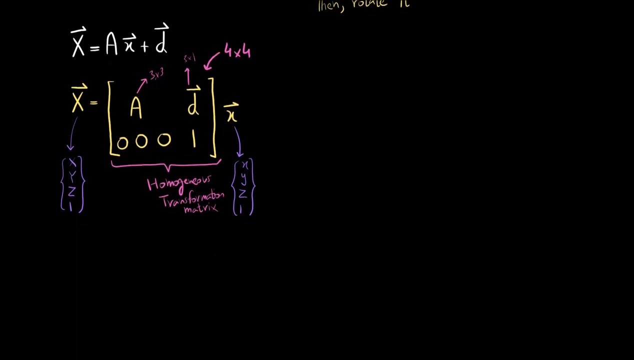 homogeneous, homogeneous transformation matrix. so what a homogeneous transformation matrix does is it enables us to do coordinate transformation. that is all that it does, so so i've written it in the short form: x equals to h times the small x, where h is my homogeneous transformation matrix. and once again, this x is not just the x, y, z code. 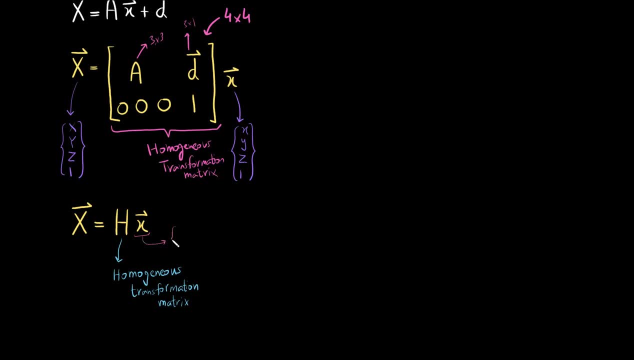 it is the x y z coordinates. in the moving frame it is the x y z coordinates. so it is the x y z coordinates and a one at the end. the one is always going to be there and this is going to be the x y z coordinates. 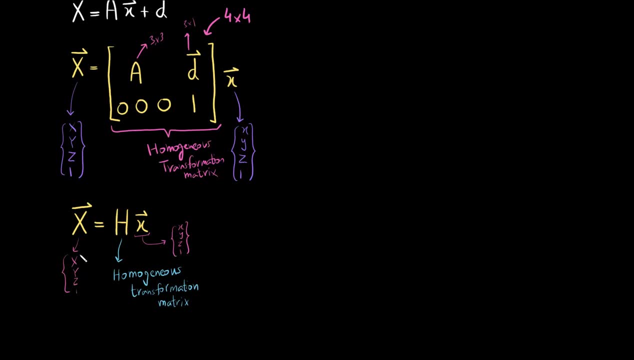 in the fixed frame, followed by a one. and why do we have that one again? because of the way that we constructed the homogeneous transformation matrix, because we had to add one extra row in order to make it a four cross, four matrix. so so that is what we did, and if you look at this again and if i just quickly multiply it out, you can see. 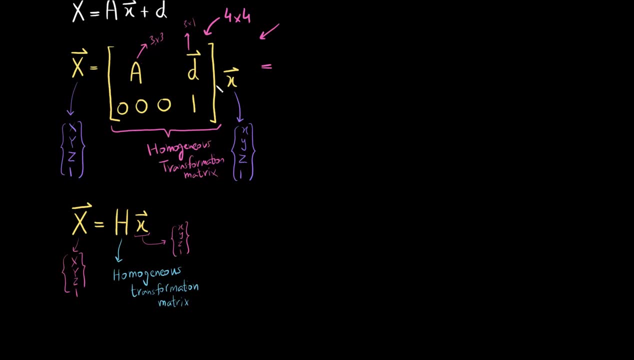 that i would get the equation on the top. so if i multiply it out, i get a times x. uh, a times x, which is this part- i'm just considering x to be this part- and then d times one. so i get this. so you can see that. 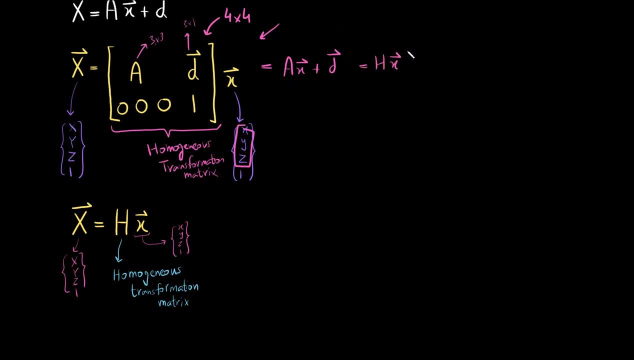 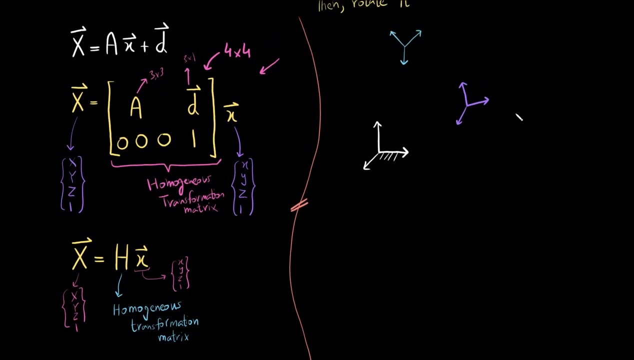 this is the same as this right, where this has a one at the end and distance have one at the end. so now the question is: why do we bother with all of this in the world of robotics? so before we talk about why we do it, and specifically for the world of robotics, let 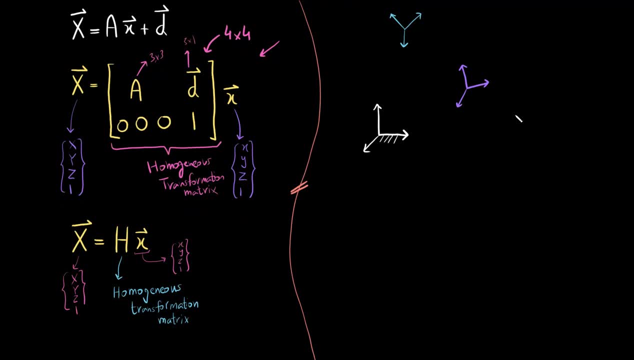 me tell you one very important and very nice property of using homogeneous transformations. so let's say, if i have a fixed frame here and there's a moving frame here and there's another moving frame here, and the thing is that i know the homogeneous transformation that takes this, 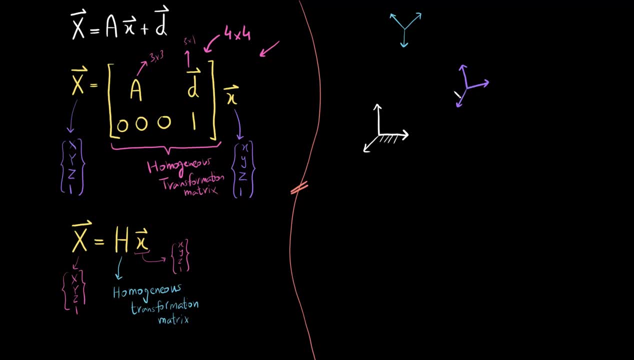 to the first moving frame and another homogeneous transformation that takes this moving frame to this moving frame. so this is what i mean. so x1 is my first homogeneous transformation and x2 is my second homogeneous transformation. now, if i need to figure out the homogeneous transformation that takes the fixed frame from the first homogeneous transformation to the second homogeneous, 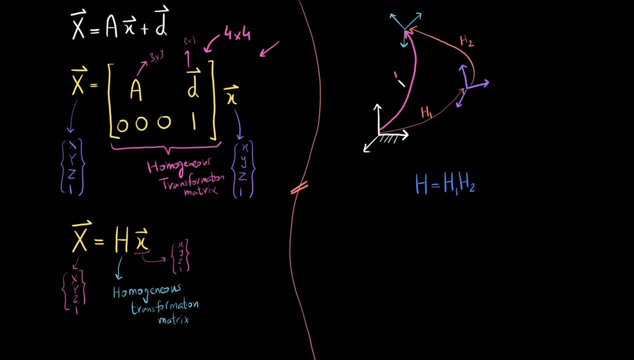 frame directly to this right? i need to find out this. so the process is very simple. all you need to do is you need to multiply the successive homogeneous transformations in this manner and you get the final homogeneous transformation, and this applies no matter how many homogeneous transformations you have. so, once again, so what we are doing is we have two moving frames and 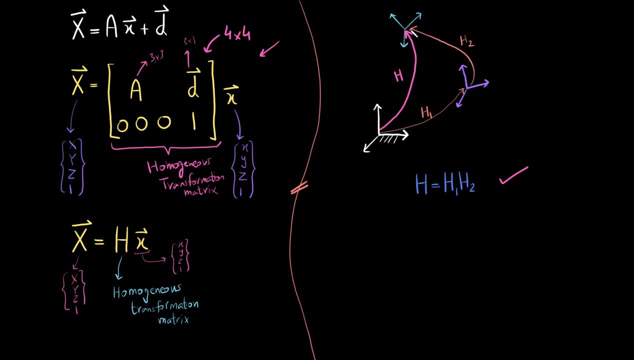 the first moving frame is expressed with respect to the fixed frame. the second moving frame is expressed with respect to the first moving frame, and we know the homogeneous transformations. so we just multiply the successive homogeneous transformations and we what we get is another homogeneous transformation matrix which is going 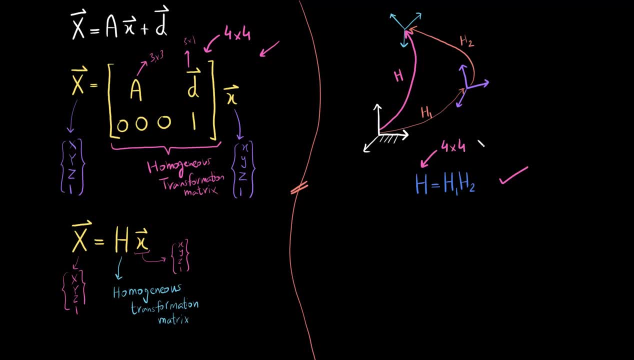 to be a four cross four matrix, which again would have the property that it would have. it would be of this form, where this: there would be a rotation matrix, 3 cross 3, there would be 3 zeros, there would be a displacement vector and then then the 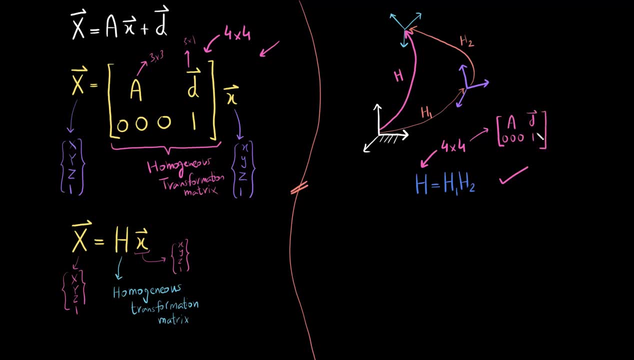 going to be a one, and this displacement vector d is what would take this point right here to this point right here, directly, and this rotation is what would like, the rotation that you would need to do after taking this frame to this uh point, in this manner, the rotation that 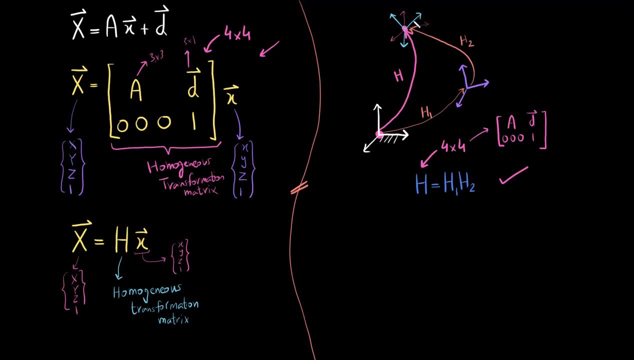 you need to perform in order to get it aligned with the moving frame. and now, if, let's say, i have a point which is defined with respect to my second moving frame, let me erase this out first. so let's say, if i have a point small x, which is defined with respect to this moving frame, 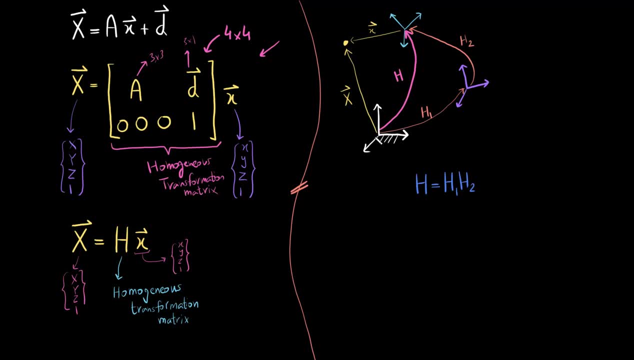 and i need to find the same point with respect to the fixed moving frame. all i need to do is i need to use this equation- x equals to x times x- and you get the answer. and similarly, there are times when you do not know the location of an object with respect to the n factor. rather, you know the location of. 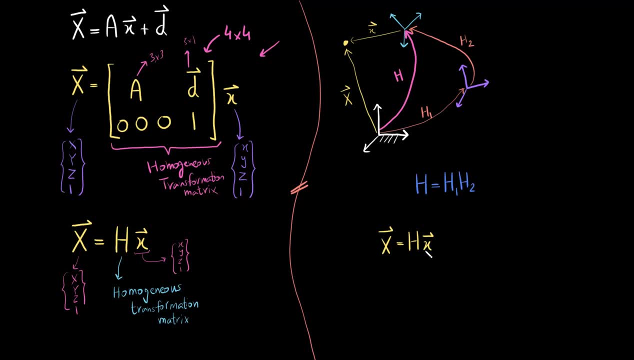 of the object with respect to the base of the robot. so all you will need to do is you would use the same equation, but what you would do is you were. so what you are going to find is the small x, which is the point expressed in the n factor frame or the moving frame. 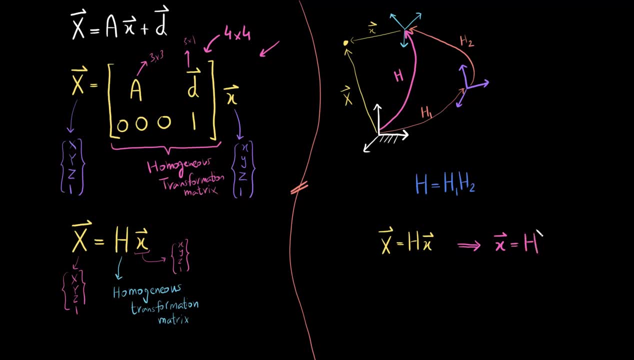 so you just take the homogeneous transformation matrix to the other side, you take the inverse and you get this and now you input. so the big x is the coordinates of the object with respect to the base of the robot and the small x is the coordinates of the object with respect to the n. 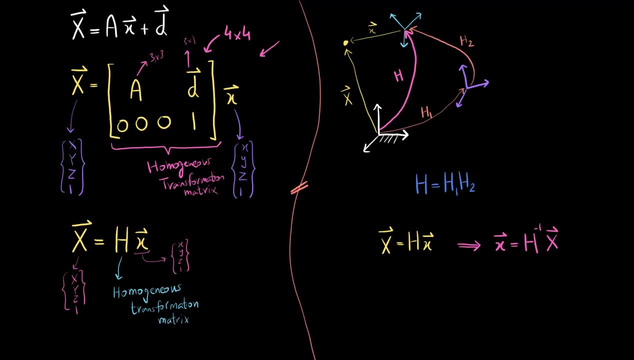 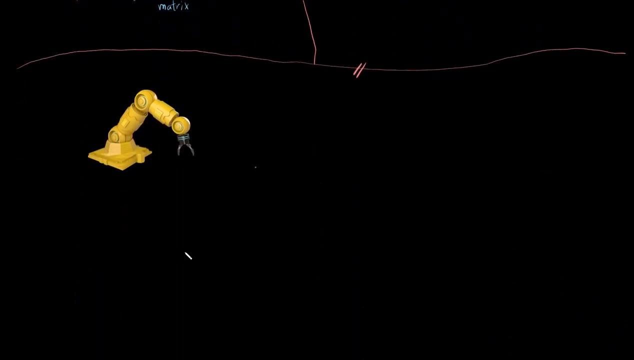 factor. we are going to deal with specific cases and we are going to work through a few numerical examples in the future couple of videos, but for now i would i do want to leave you with, uh, a better understanding of what we have done. so let's say i have a robot here which is a a normal 3d robot which has a revenue joint here. 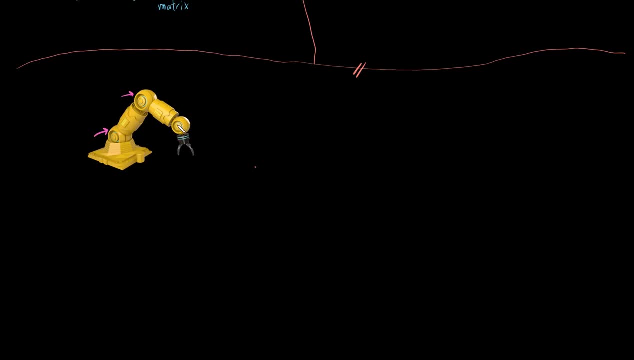 a revenue joint here, a revenue joint here. right, and now we have two, uh, reference frame. the first is, let's say, the first is this one. let me use another color, okay, so the first is this one. so this is my fixed frame, which is at the base of the robot. 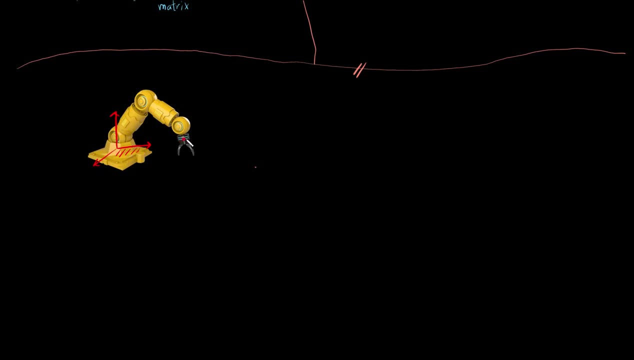 and then i have another uh frame, which is the moving frame. let's say, i have the moving frame, this, this and this. okay, so this is my moving frame and this is my fixed frame. and now i need to figure out the homogeneous transformation that takes the fixed frame. 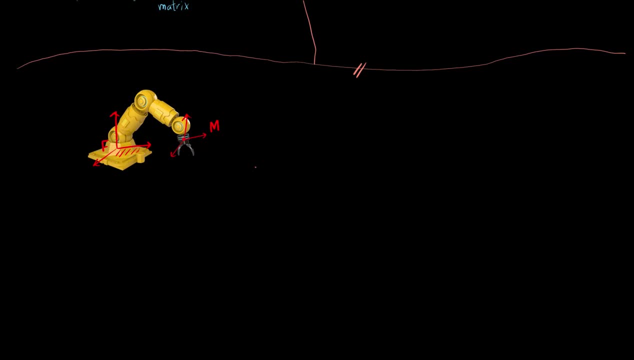 to the moving frame. so what i would do is, first and foremost, i would figure out the homogeneous transformation that takes this fixed frame to this um joint, so i call it as h1, and then i need to figure out the homogeneous transformation that takes this frame to this point. 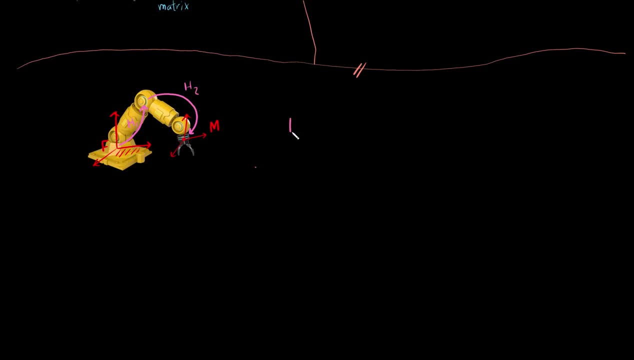 h2, and once i get h1 and h2, i can just simply find h, which my h is this, which takes the fixed frame directly to the moving frame. so my h is going to be equal to the first homogeneous transform multiplied by the second homogeneous transform. 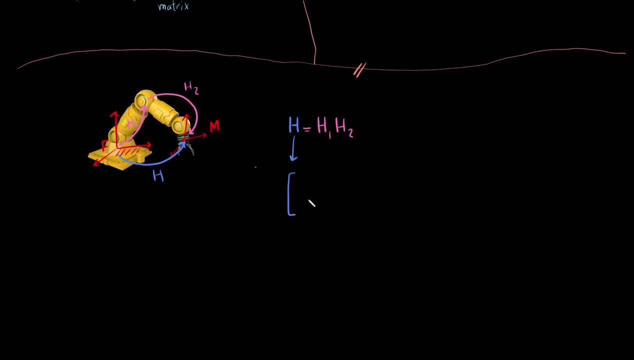 and once again, this h is going to be of the, of this form a, and then there are going to be three zeros, so i can shorten them up by writing this zero vector transform and there's going to be a displacement vector, and then there's going to be a one, and this displacement vector, right here, what?